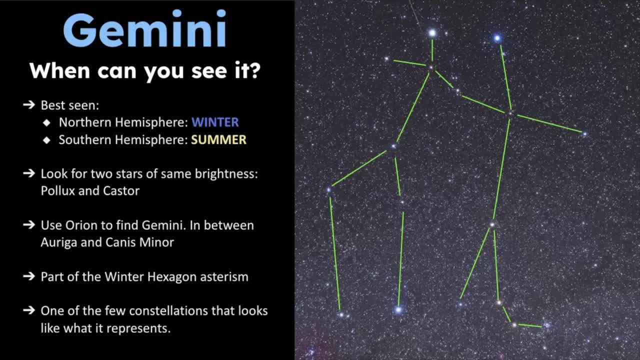 see Gemini. during this time. You want to look for two stars of similar brightness, and that would be Pollux- right here- and Castor. You want to also use Orion to help you find Gemini, and oftentimes I will use Auriga and Canis Minor to help me find Gemini as well. It is part of the winter hexagon. 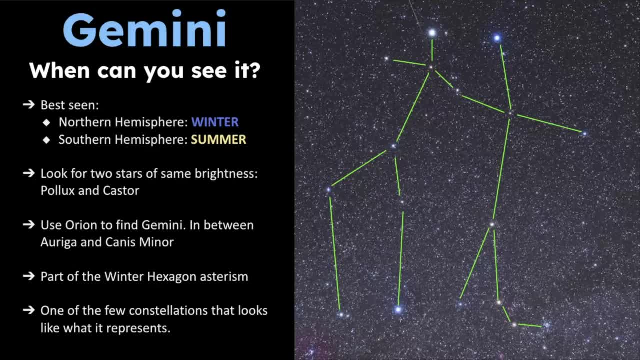 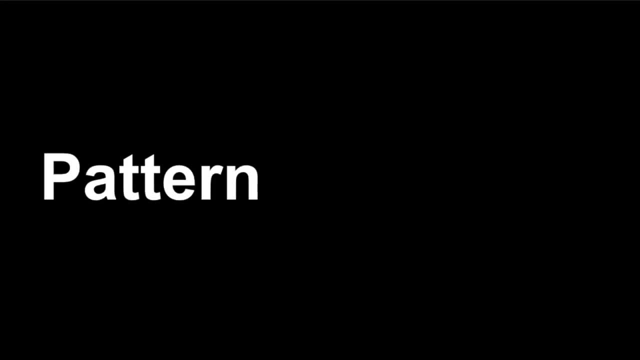 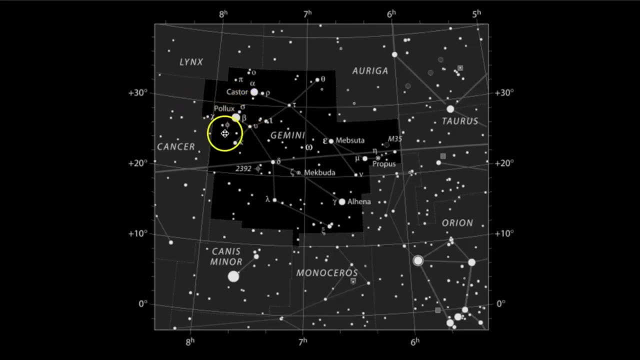 asterism, which we will take a look at later on in this video, And I do think that it's one of the most important stars in the calendar because it looks like what it actually represents. Let's examine the pattern that Gemini makes in the sky. Here we have an official star map of what a 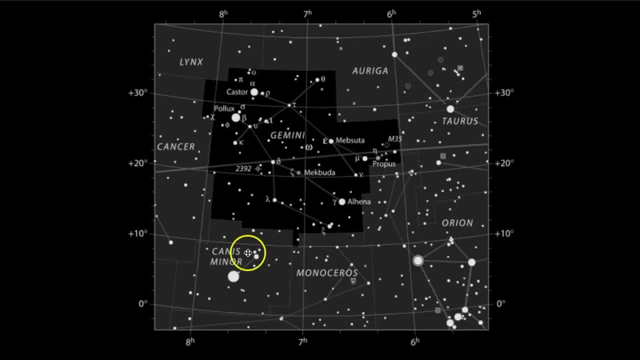 Gemini looks like, and you'll probably notice the two bright stars here, Castor and Pollux. There are some other bright stars around, such as Procyon and Canis Minor. You have Orion nearby, as well as Taurus and Auriga, So let's take a look at some pictures and see if we can connect the map to what this pattern looks like in the sky, So Gemini is right in the center of this photograph and notice that Castor and Pollux shine brightly together. They are different colors, though, even though their magnitude is fairly similar, And if we were to point out where the pattern is, this is what. 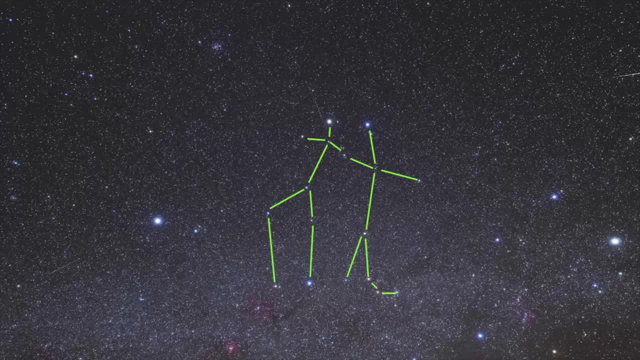 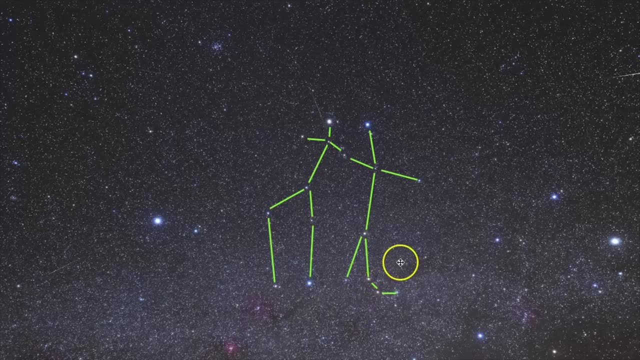 Gemini looks like in the sky. Now the trick I teach my own students in the classroom on how to remember the difference between the two is that Castor appears to have a cast of two stars, So I have a cast on his leg. In my first year of teaching, I had a student come up with that, so I 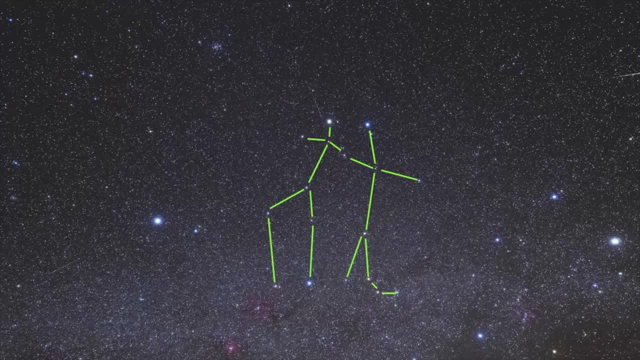 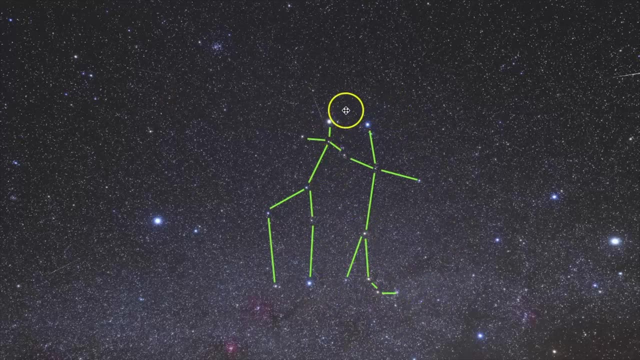 can't truly take credit, but I am thankful for this way to help me remember the difference between the two. So Castor is here with the cast on his leg and Pollux is right here Now. in terms of other constellations that sit nearby, we have a few. Right here is Canis Minor. that's represented as 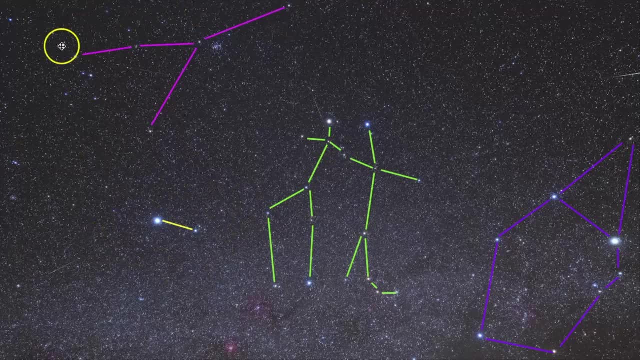 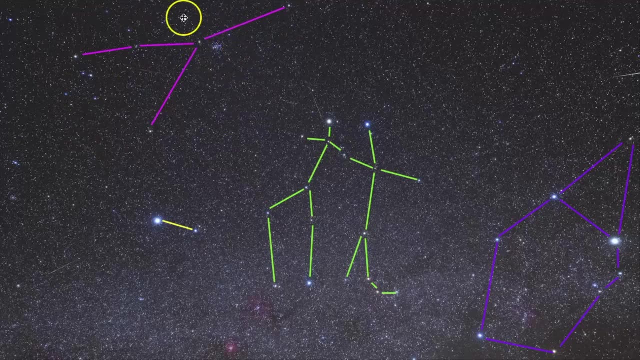 the small dog, and up here is Cancer, And you can tell it's Cancer because it's a small dog and it's a little star cluster right here that's known as the Beehive Star Cluster And it's really the only way I can find Cancer. But over here you have Auriga- or some people pronounce it Auriga- And 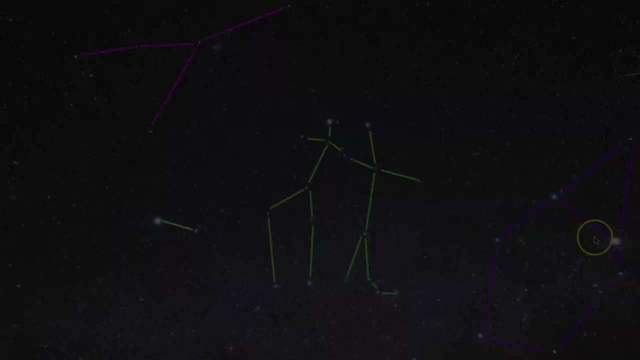 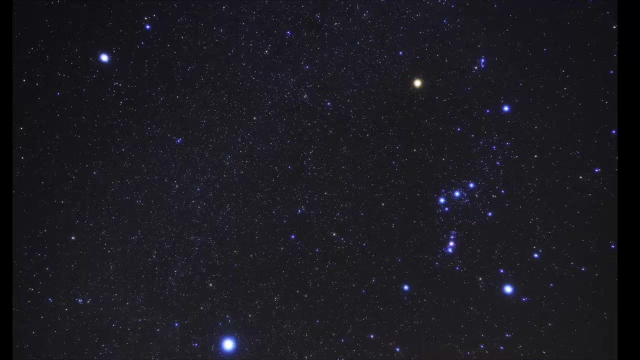 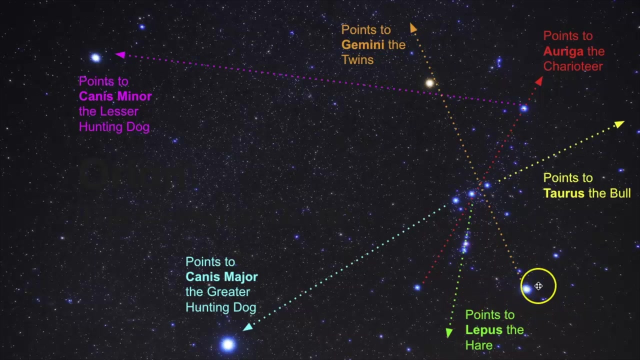 this star right here is known as Capella. Another great way to find Gemini is to use Orion to help you out. Orion is really the guide to all of this area of the sky. So if you look at Orion, you want to find Rigel and then draw a line from Rigel through Betelgeuse and that will point towards. 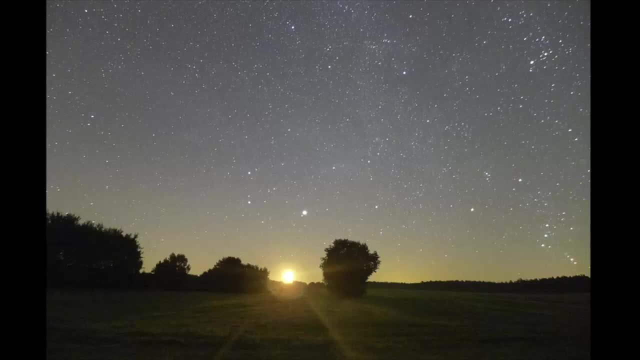 the twins. Let's get some practice at this. So here, if you're looking at this photo, take your eyes to the bottom right, and that is where Orion is Now. find Betelgeuse or Betelgeuse. there's multiple ways. 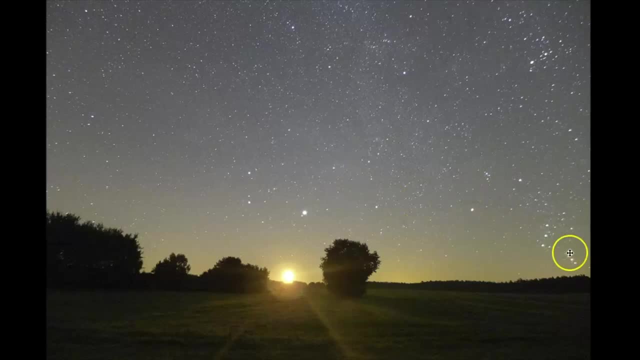 to pronounce that star, which is right here. You can draw that line to guide you right to Gemini. So if we were to point everything out, this is where Gemini is- And notice that the orientation of Orion is different than that of Gemini. It's like if Orion were standing upright. Gemini seems to be tilted onto its side, And this 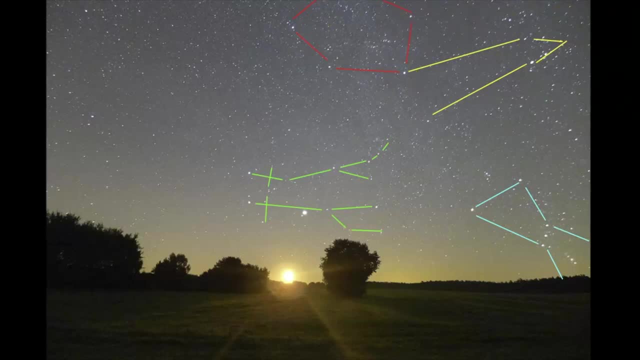 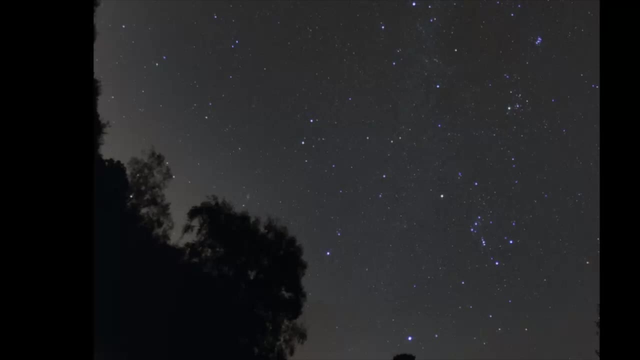 here is Taurus and this is Auriga. Let's get a little bit more practice using Orion. So hopefully you can find Orion towards the right side- maybe midline to bottom part of this photograph- and then find Rigel, Draw a line to Betelgeuse and that is where Gemini will be. And if we were to point everything out, this: 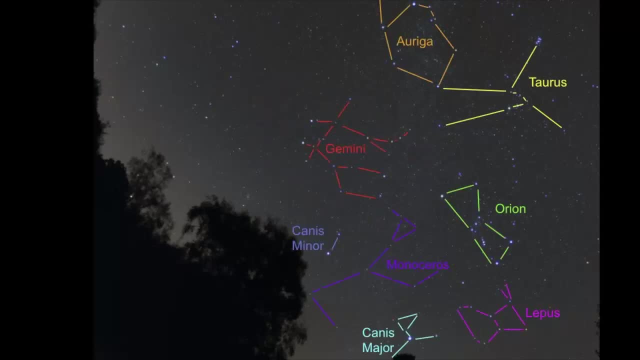 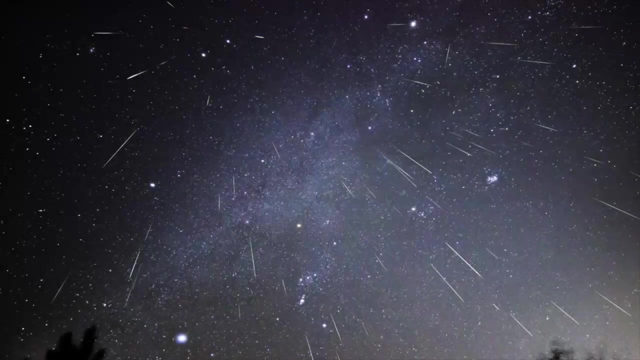 is what this area of the sky is like. You can also use the winter triangle to help you find where Betelgeuse is in Orion, and then right there is where Gemini is. Gemini is also part of the winter hexagon- asterism. 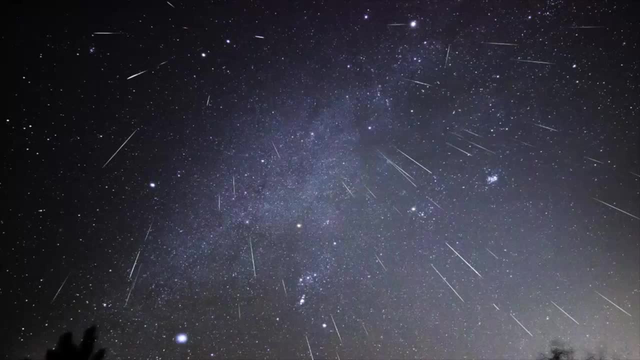 And this looks like a busy picture, But if you can just notice the stars in the sky, the stars in the sky are very active. the background instead of the meteorites. that's what we're going to focus on Here, is what the 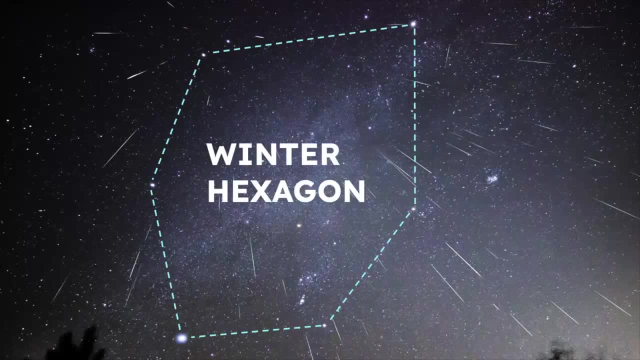 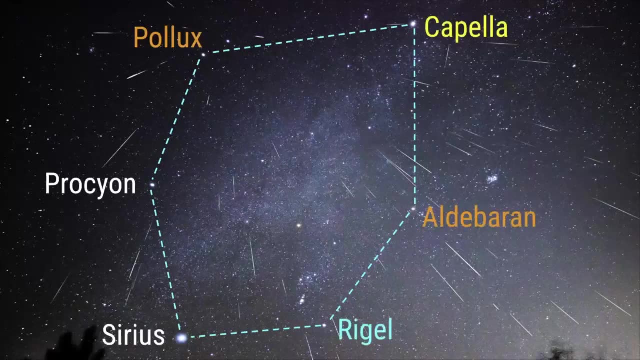 winter hexagon asterism looks like, and it is made up of the six brightest stars in this area of the sky, And those stars include Pollux, and Pollux is in Gemini. We have Capella, a part of Auriga. Aldebaran, which is part of Taurus. Rigel, which is the foot of Orion. Sirius, which is the brightest. 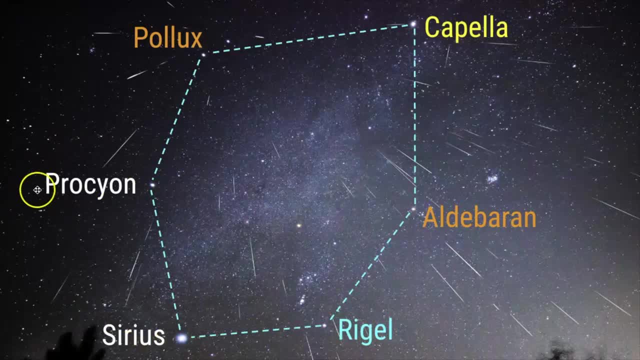 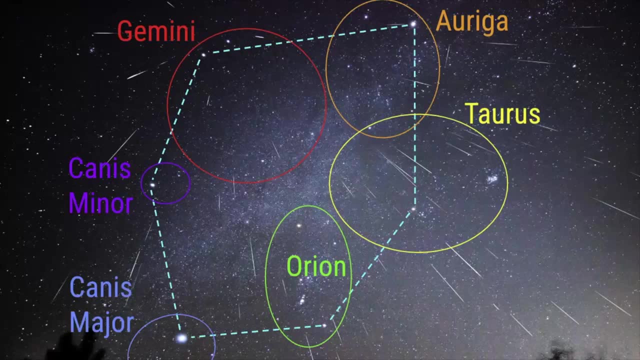 star in Canis Major and Procyon, which is the brightest star in Canis Minor. And if we were to point out where all those constellations would be, this is where Gemini is. Auriga is kind of like a pentagon-shaped pattern. Taurus is right here, Orion is very obvious because of the belt. 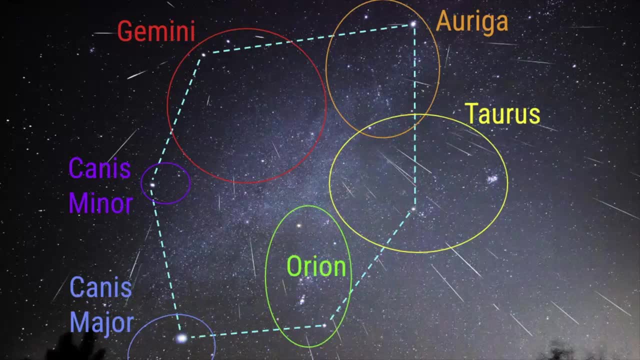 stars. Canis Major is easy to find because Sirius is the brightest star in the night sky, And then Canis Minor is just a simple two-star constellation. Sometimes it could be confused with the heads of Gemini, but I don't ever confuse them because I 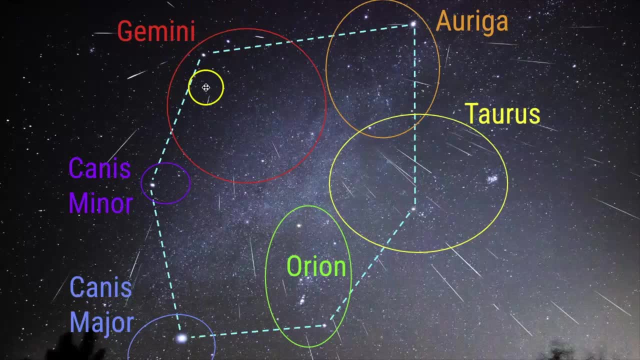 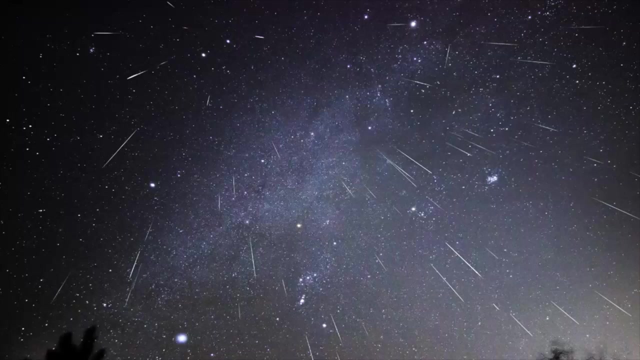 know that the two stars of Gemini are of pretty much of equal brightness. And again, this picture. what's really cool about this is it was taken during the Geminids meteor shower and that is the most prolific meteor shower of the year and it usually peaks mid-December. I do have a video. 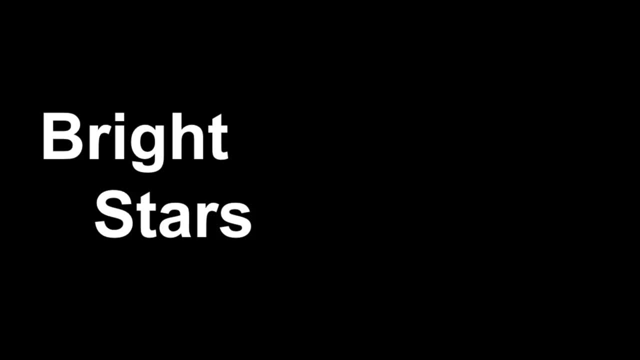 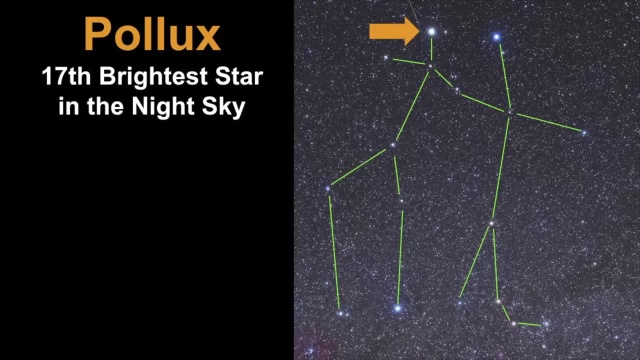 about it, so go check it out. Now let's take a deeper dive into the brighter stars of Gemini. We begin with Pollux, which is the brightest star in Gemini. However, it's the 17th brightest star in the entire night sky. Pollux is classified as an 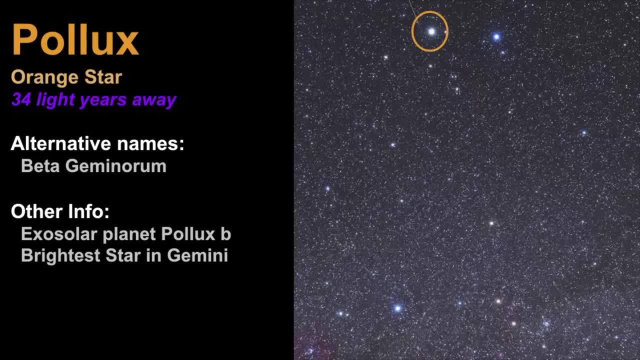 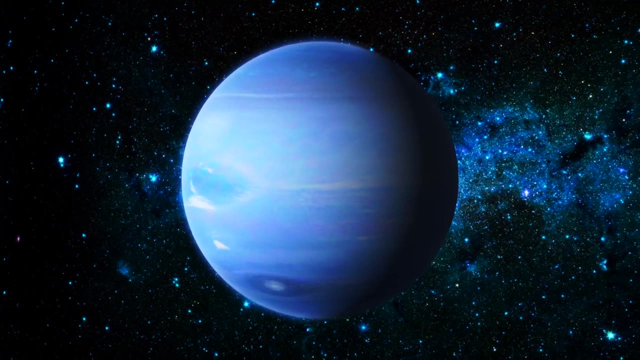 orange giant star, and it's estimated to be 34 light-years away. It's already fused the hydrogen inside its core and now it is currently fusing helium and expanding in size. It does have an exosolar planet that orbits around it, called Pollux b. 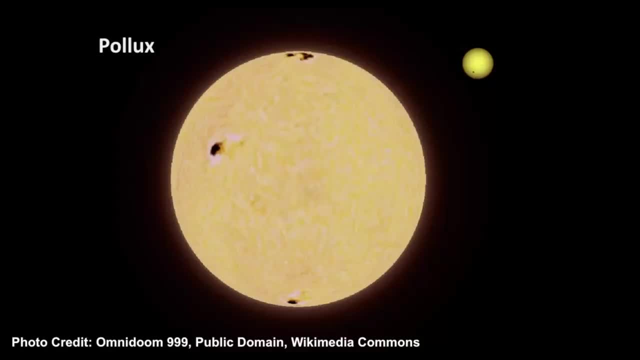 Now, when you look at the size comparison between the Sun and Pollux, Pollux only has about two times more mass than our own Sun, but it is much bigger in size. You could fit nine Earths across the diameter of Pollux. 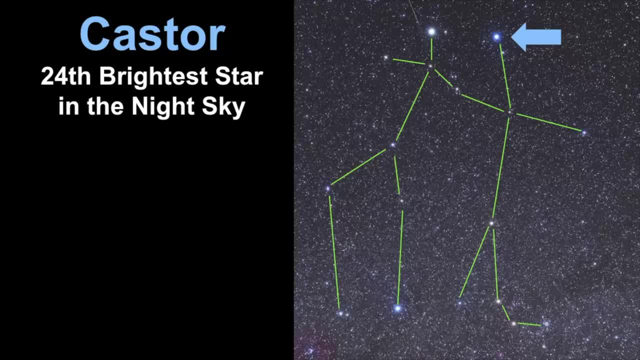 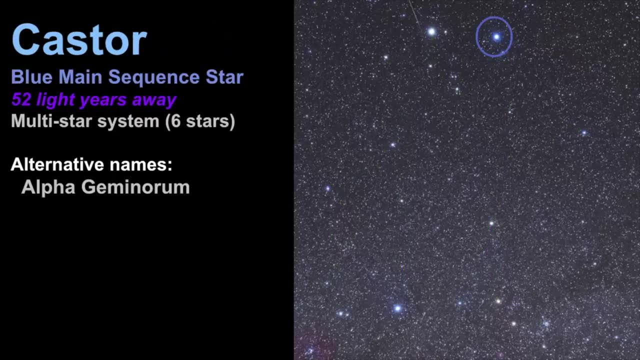 Castor is the 2nd brightest star in Gemini, but overall it's the 24th brightest star in the night sky. It's classified as a blue main sequence star and it's estimated to be 52 light-years away. It is a multi-star system consisting of three binary pairs. 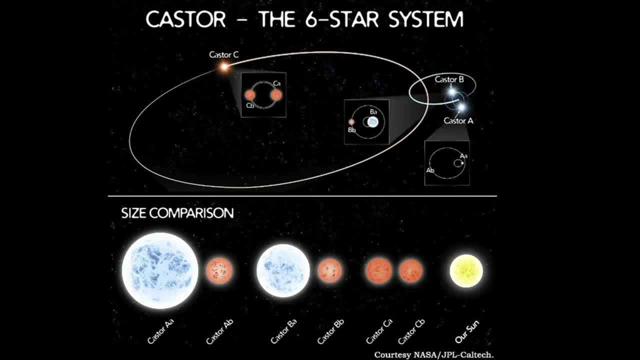 When we break this down you can see the castor A system is a blue mean sequence star and a red dwarf star. That's the same as the castor B system, but castor C consists of two red dwarf stars And when you look at all of these stars together, notice the size comparison to our own home star. 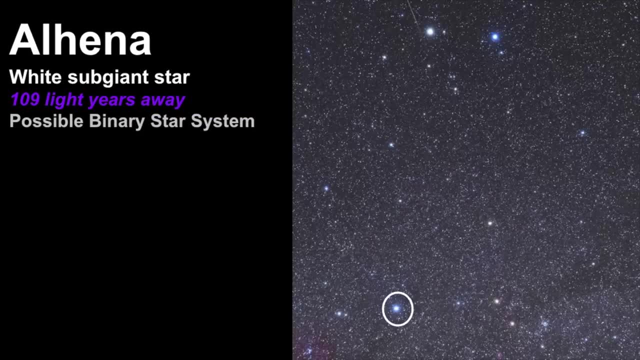 Alhena is the third brightest star in the constellation of Gemini and it's classified as a white sub-giant star. That means it's run out of hydrogen in its core and it's starting to fuse helium and grow in size. It's also a possible binary star system and it's estimated to be 109 light-years away. 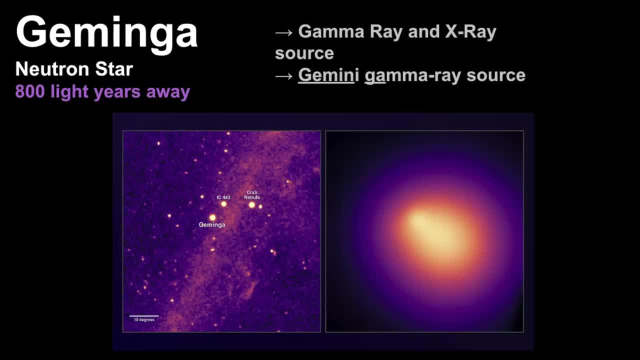 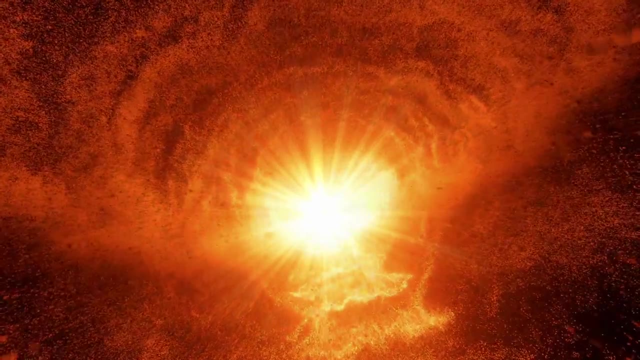 Another cool star I learned about in Gemini is called Jaminga. It was discovered in 1972. It's a neutron star that's estimated to be 800 light-years away and it's among the brightest pulsars in the sky. Remember a pulsar or a neutron star is the crushed core left behind when a star that is much more massive than our own sun ran out of fuel. 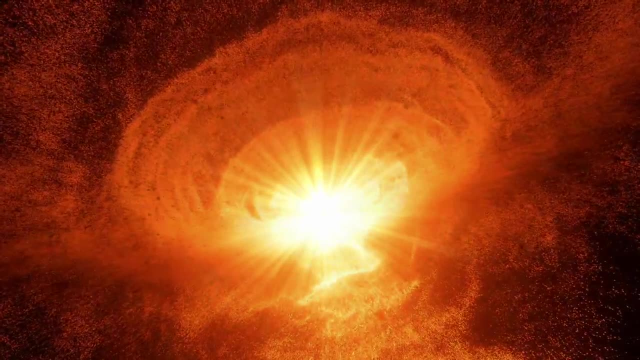 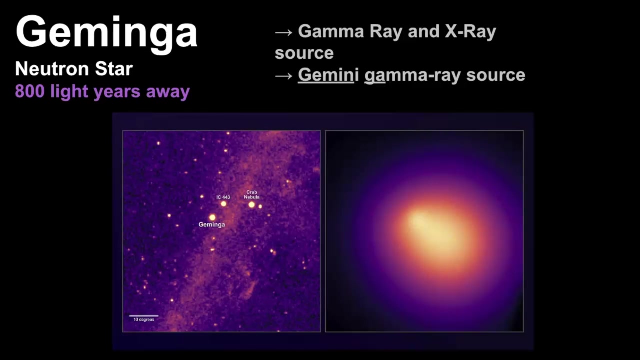 collapsed under its own weight and then turned into a supernova. So here in this picture, what you're looking at is the halo around the pulsar. Let's break this down. Let's review some of the celestial objects that are located in the boundaries of Gemini. 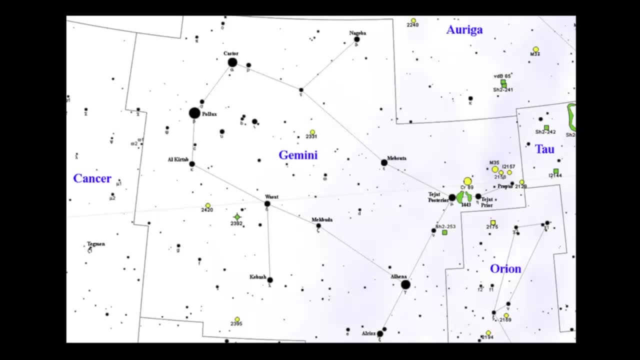 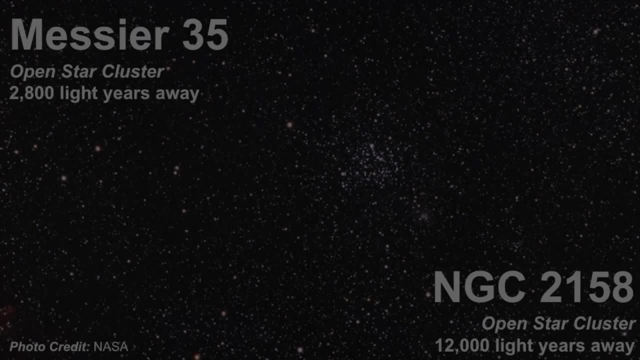 Gemini is a great place to look for different celestial objects and there are a variety of objects you can see, such as open star clusters and a few nebulae. Messier 35 is an open star cluster estimated to be 2,800 light-years away. 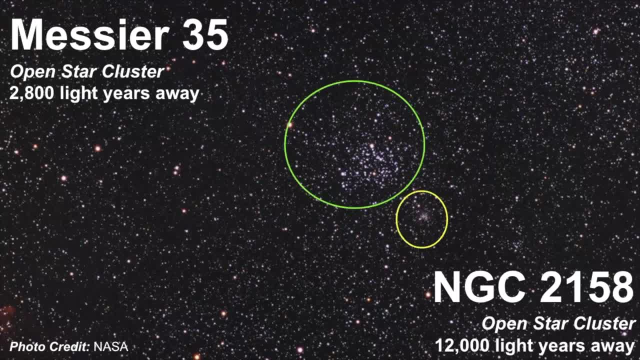 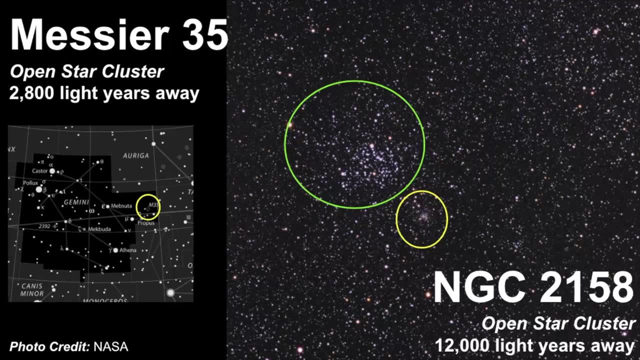 and situated right next to it is another small open star cluster. It's called NGC 2158, and its distance is It's estimated to be 12,000 light-years away, and when you're looking in Gemini, you want to look for the area in Castor's cast. 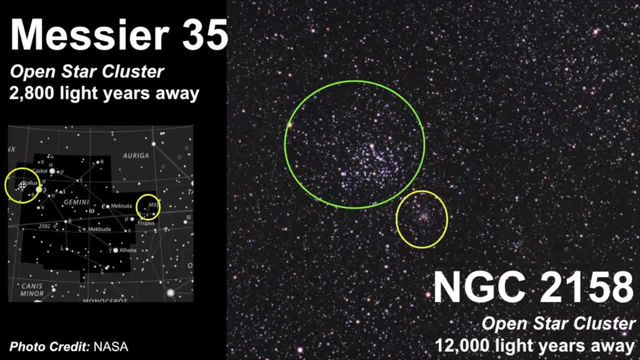 Remember I taught you that trick- to remember which one is Pollux and Castor. Castor has a cast on his leg and that's where M35, or Messier 35, will be. What I like about this open star cluster is that it has a magnitude of 5,, so if you're in areas that have very dark skies, you should be able to see it. 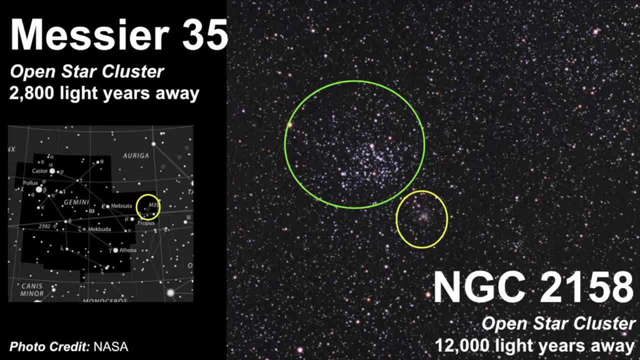 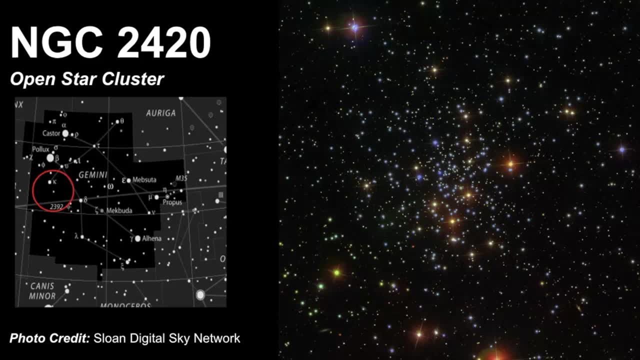 And if you're going to use anything to get a closer look, binoculars would be best. Another object to see is called NGC 2420, and this is an open star cluster located on the Pollux side of Gemini. In the same area is the Eskimo Nebula. 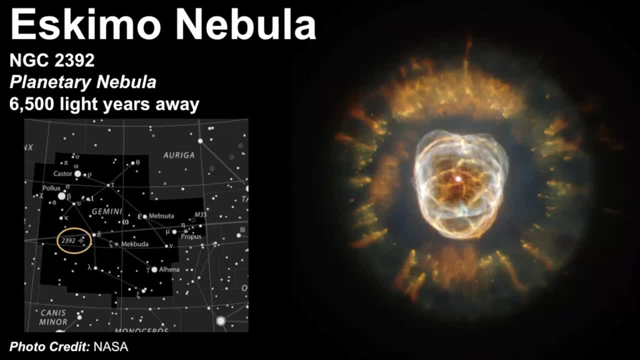 It also has the name NGC 2392, and this is a planetary nebula, which means it's a star that is no longer fusing any hydrogen. It's actually the leftover layers of a dying star. so inside here is a white dwarf, and then here there are two different sets of rings that surround it. 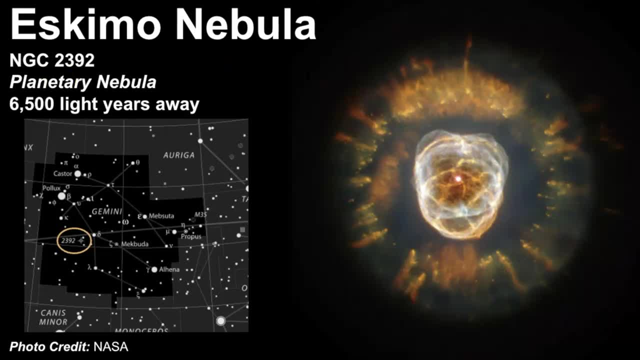 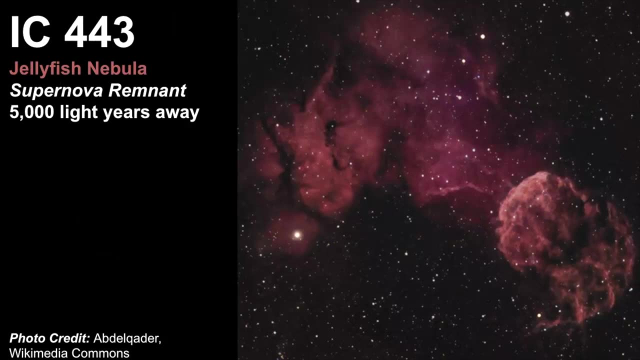 And when you're looking for this celestial object, you want to look towards the hip of Pollux, and that's where you're going to find the Eskimo Nebula. Another nebula to look for is called IC 443.. It's nicknamed the Jellyfish Nebula and it's a supernova remnant. 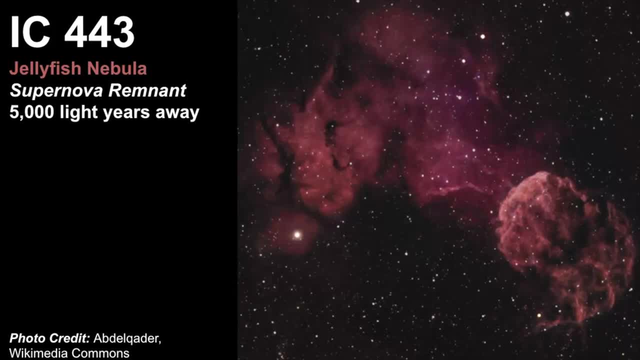 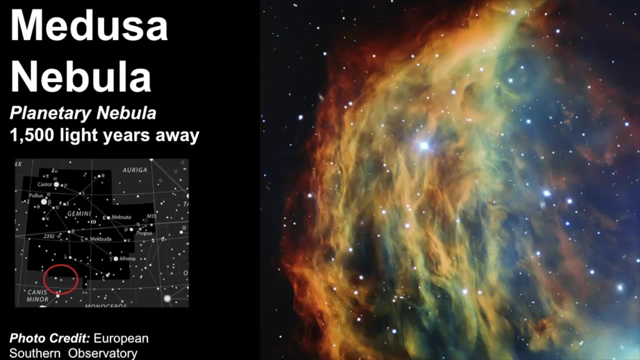 Which means that it's a star that has exploded long ago, and then the shell of that explosion is still expanding. It's estimated to be 5,000 light years away. Another beautiful object to spot is something called the Medusa Nebula. 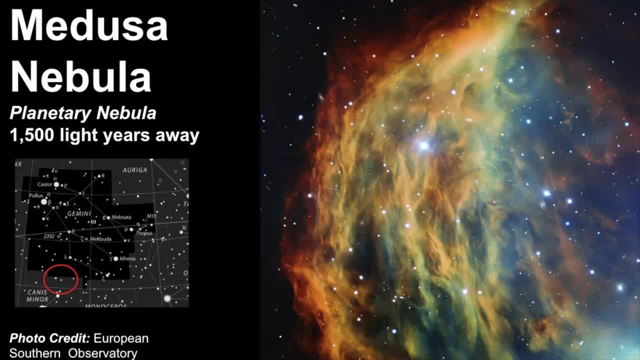 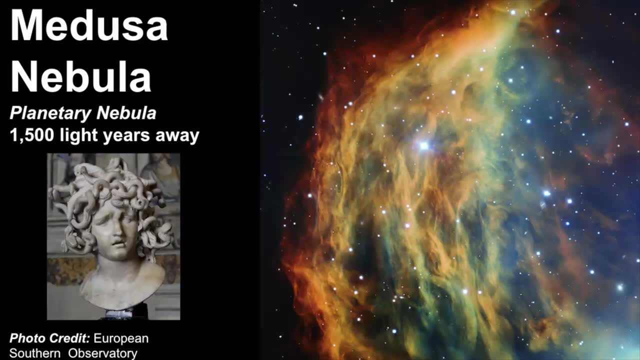 This is also a planetary nebula that's estimated to be 1,500 light years away And it's right along the border between Canis Minor and Gemini, And it gets its name after the Greek mythological creature known as Medusa, because the filaments of glowing gas tend to look like the serpent hair of Medusa. 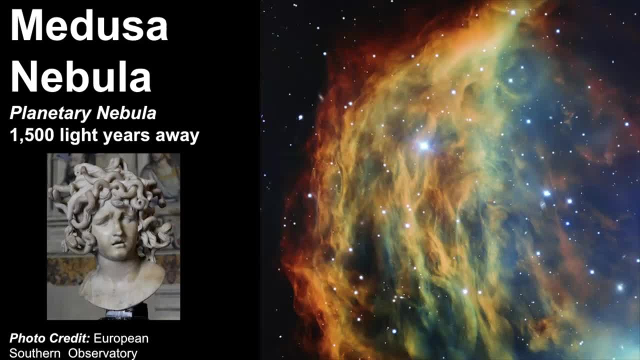 Now this is a large planetary nebula. It used to be classified as a supernova remnant, but after further study it was found to be a planetary nebula, So the star in this system is at the end of its life. 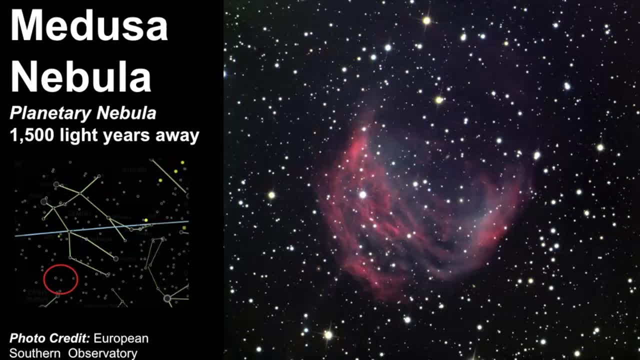 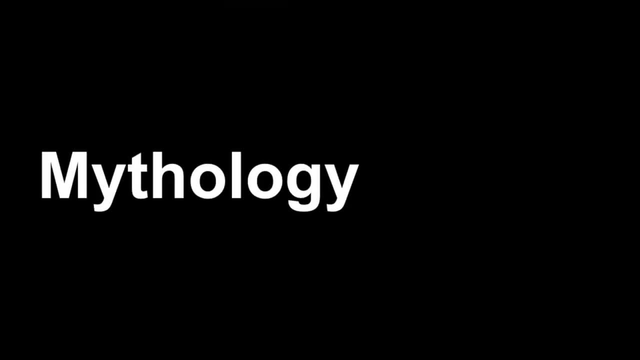 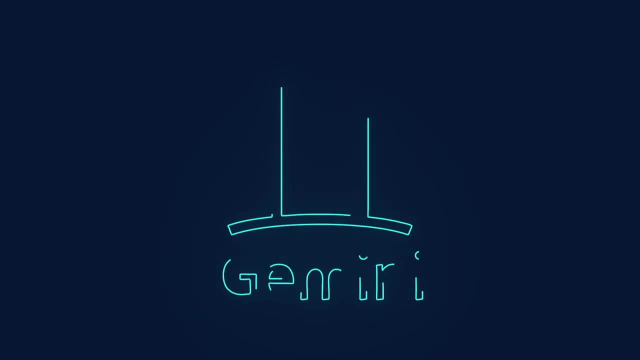 And these are the last Outer shells of the star that are just kind of being ejected away from the main core. Let's examine some of the legends behind Gemini. It is often the stories of the stars that we can connect to in some way. that can help us remember the constellations. 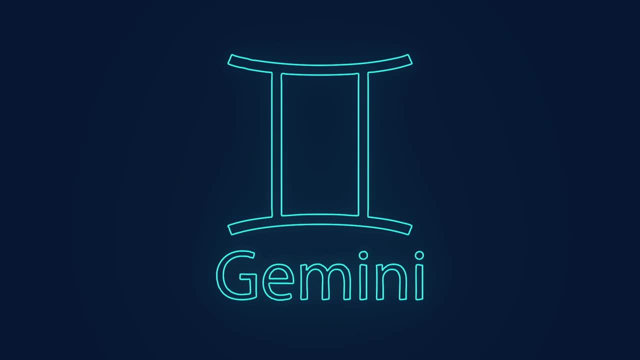 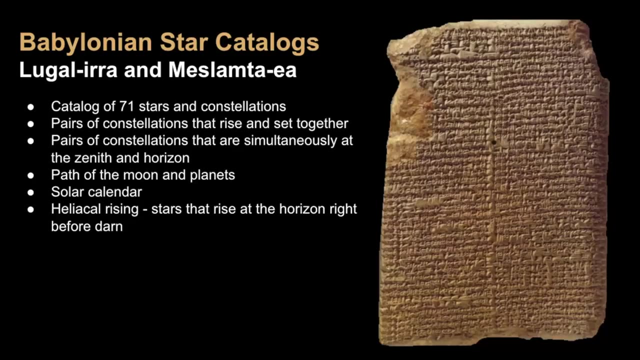 And remember there are lots of mythologies out there, so there is no one true legend for any constellation. Now, in terms of Gemini, we begin with the Babylonian star catalogs. like many of the ancient constellations, This is the names associated with Gemini. 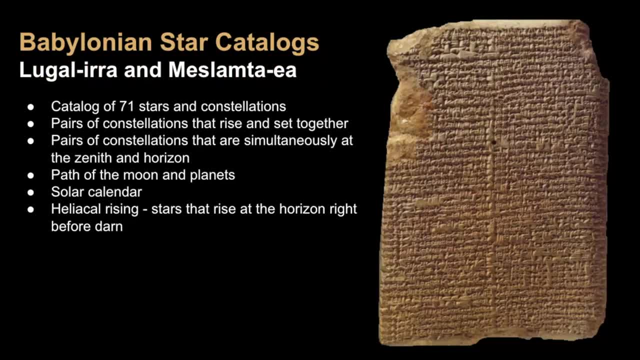 I'm not going to attempt to pronounce them- I definitely would get it wrong, but these two legends were a set of twin gods and they were identical when they were being displayed. They were shown wearing horn caps, holding axes- an axe and a mace- and they were identified as the constellation Gemini. 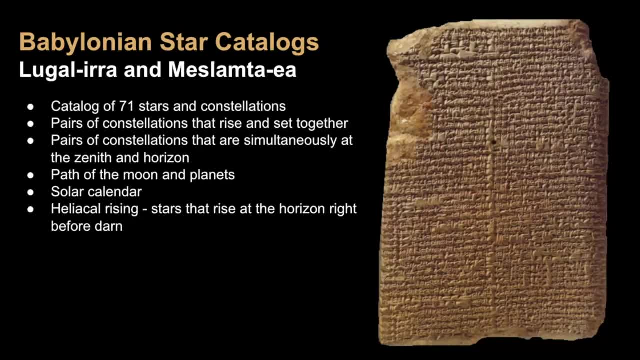 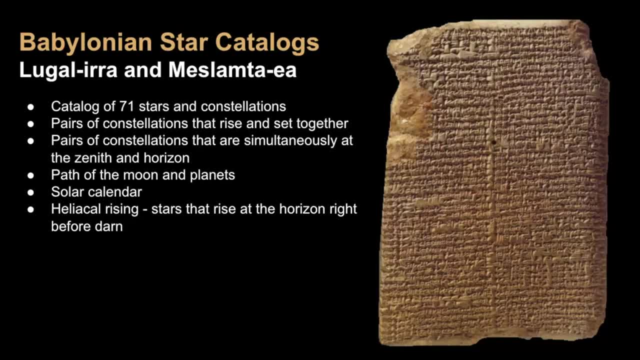 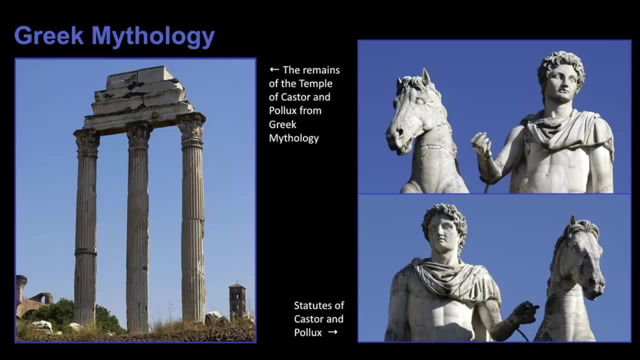 So the stars were an important guide to many things that happened on Earth. In Greek mythology, the twins are often referred to as Castor and Pollux, and both twins were hatched from an egg after their mother, Leta, was seduced by the Greek king of the gods. 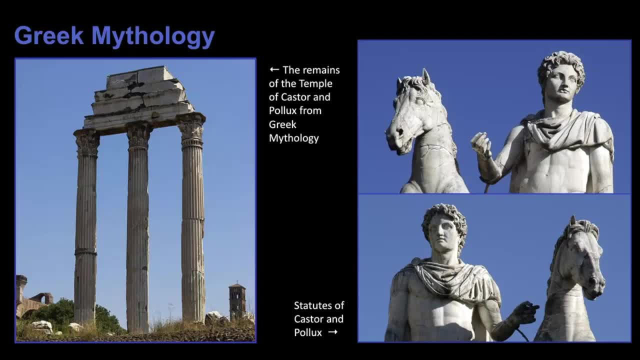 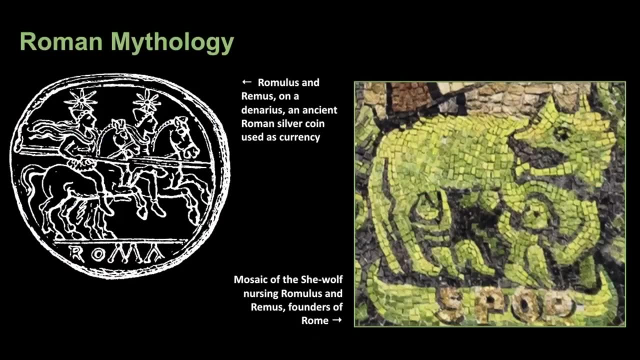 Zeus was the son of Pollux, where Tendarius was the son of Castor, And there are many ancient legends that go along with this. In terms of Roman mythology, Romulus and Remus. that is seen right here on a Roman coin. 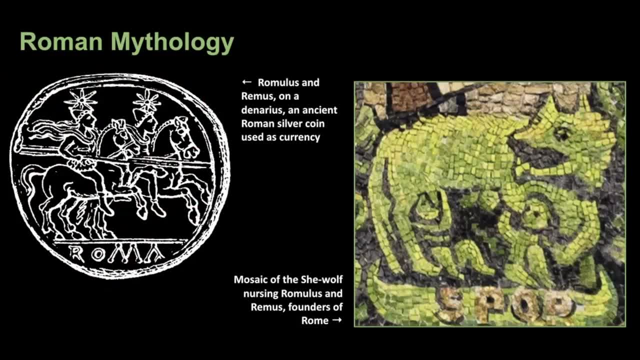 This has also been connected with Gemini And these twins have been the symbol of Rome in ancient times and very recognizable icons in ancient mythology. But of course you must remember that the mythologies of the stars vary according to time, place and culture. 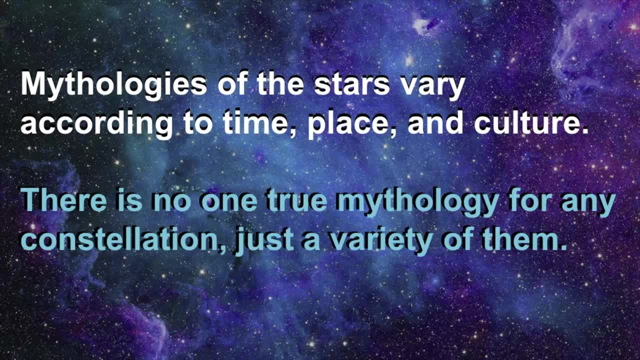 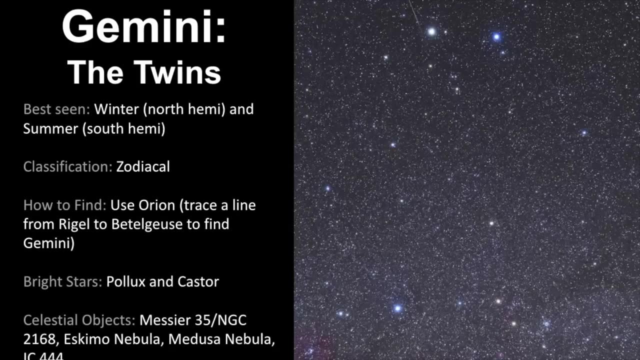 There's no one true mythology for any constellation, but just a variety of them, So let me know in the comments below what kinds of legends and mythologies live in your area of the world. Share them in the comments below. We've come to the end of our video about Gemini, So let's review everything we've learned so far. 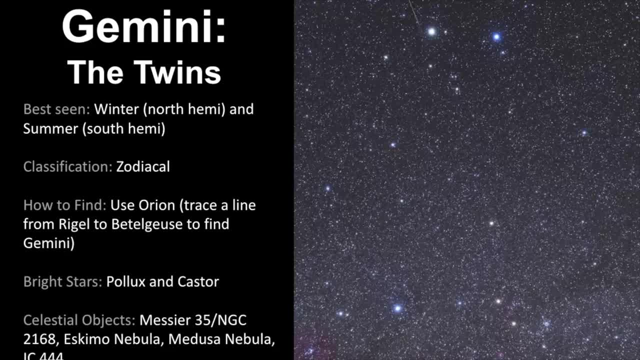 It's best seen in the wintertime for the northern hemisphere, but summertime for the northern hemisphere. It's classified as a zodiacal constellation, which means that the sun passes through its boundaries. The best way to find Gemini is to use Orion. You want to trace a line from? 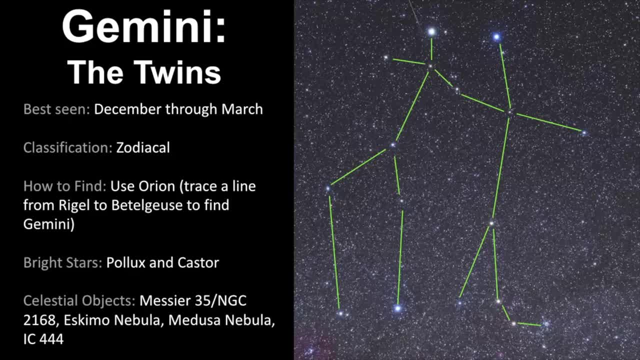 Rigel to Betelgeuse, and that will aim you in the direction of where Gemini is. The bright stars of this constellation are Pollux- right here- and Castor. Remember that Castor has a cast on his leg and that's the best way to remember the difference between the two brothers.